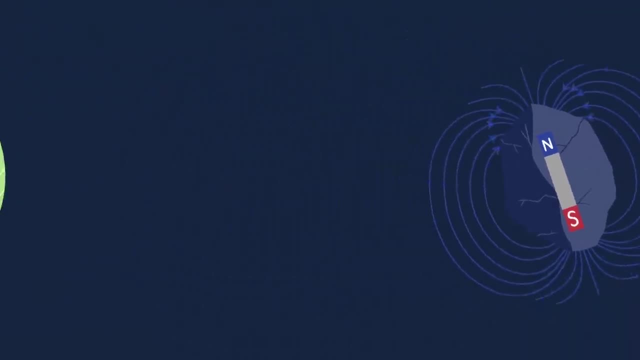 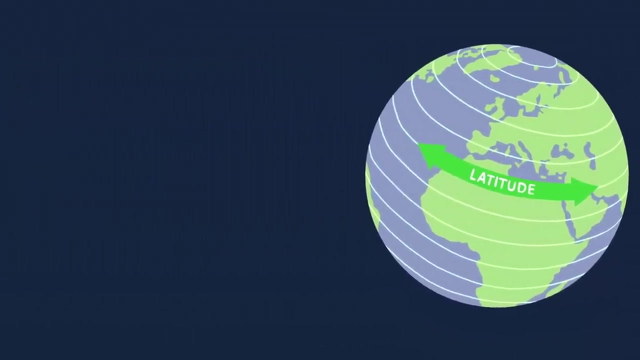 So by calculating the direction and intensity of a given rock's magnetic field, we can discover the latitude at which it was located at the time of cooling. But this approach has serious limitations. For one thing, a rock's magnetic field doesn't tell us the plate's longitude. 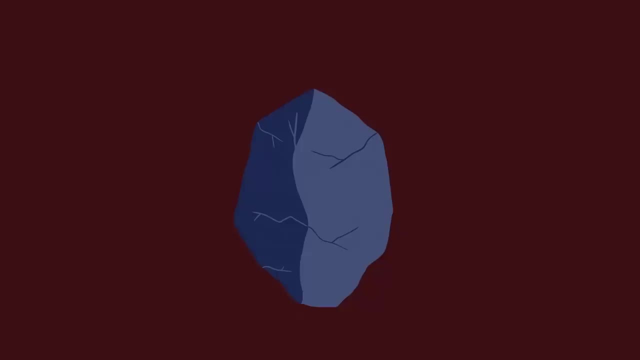 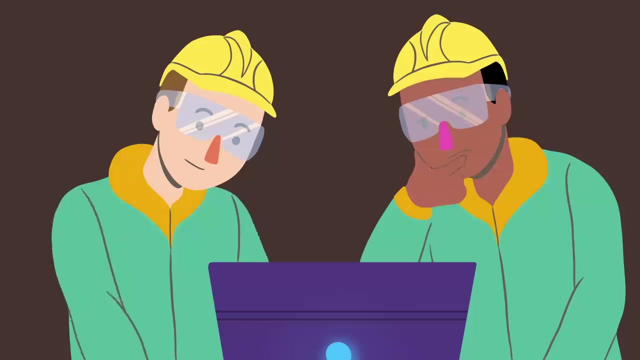 and the latitude measurement could tell us that It would be either north or south. Worse still, this magnetic data gets erased when the rock is reheated, like during continental collisions or volcanic activity, So geologists need to employ other methods to reconstruct the continent's positions. 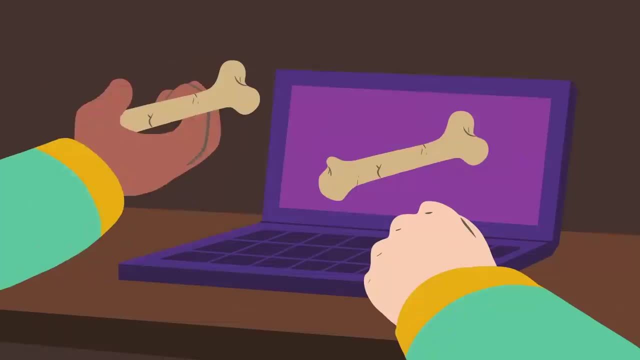 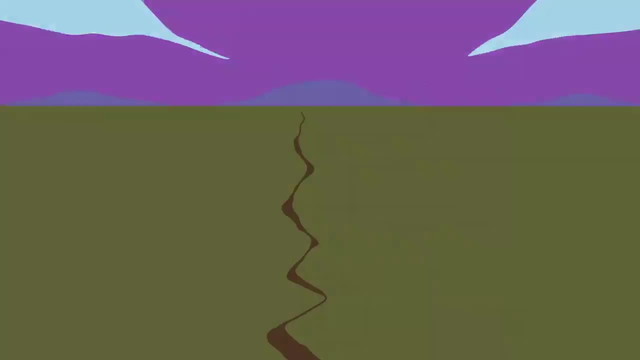 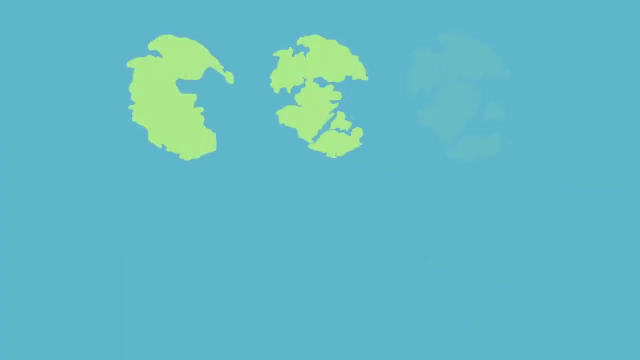 Dating local fossils and comparing them to the global fossil record can help identifying previously connected regions. The same is true of cracks and other deformations in the Earth's crust, which can sometimes be traced across plates. Using these tools, scientists have pieced together a relatively reliable history of plate movements. 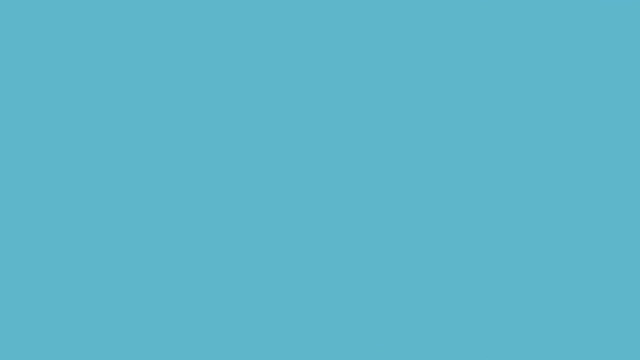 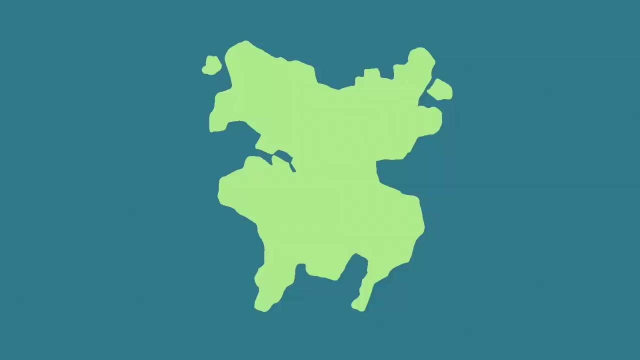 and their research revealed a pattern spanning hundreds of millions of years. What's now known as the Wilson Cycle predicts how continents diverge and reassemble, and it currently predicts the next supercontinent will form 50 to 250 million years from now. We don't have much certainty on what that landing will be. 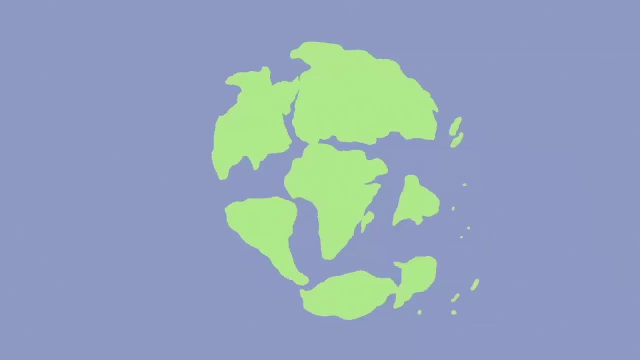 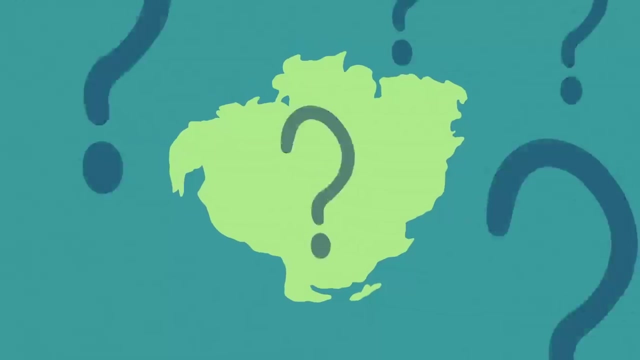 or what that landmass will look like. It could be a new pangea that emerges from the closing of the Atlantic, or it might result from the formation of a new pan-Asian ocean, But while its shape and size remain a mystery, 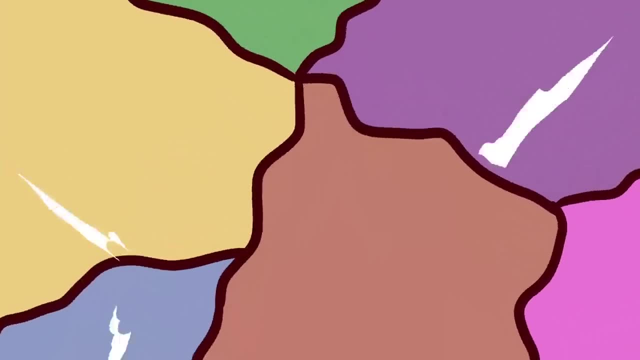 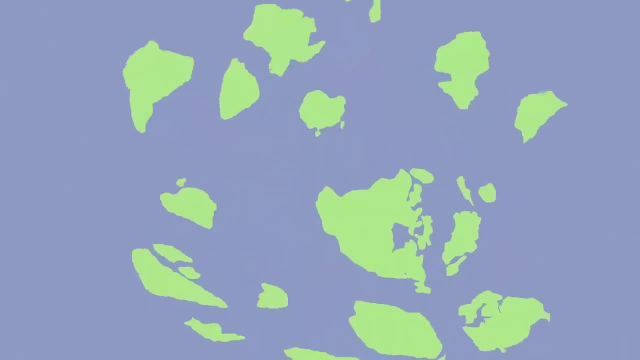 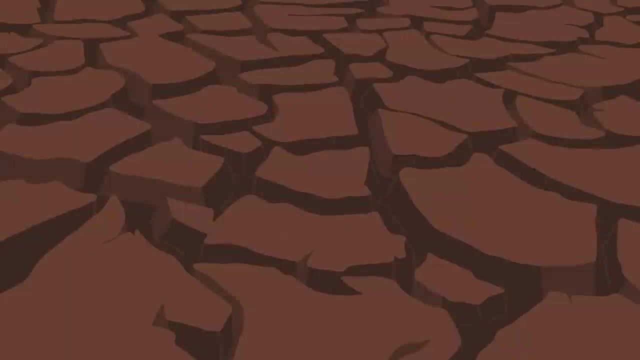 we do know these changes will impact much more than our national borders. In the past, colliding plates have caused major environmental upheavals. When the Rodinia supercontinent broke up circa 750 million years ago, it left large landmasses vulnerable to weathering. 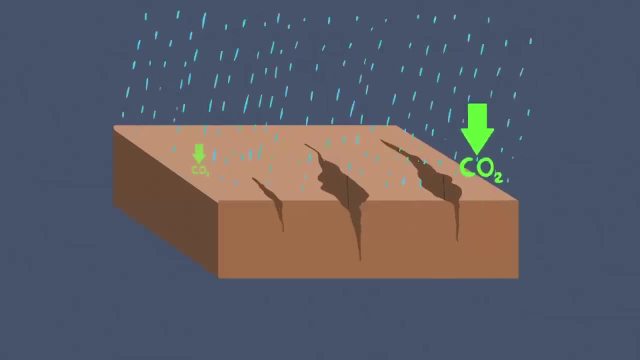 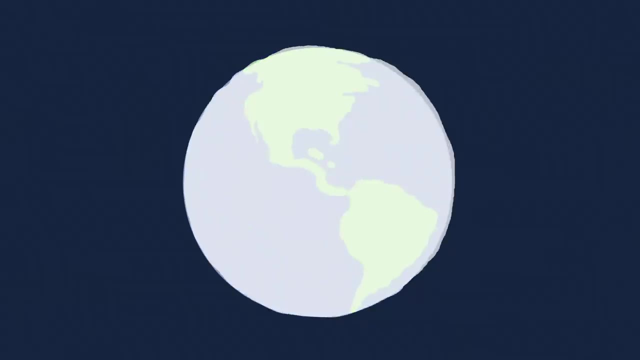 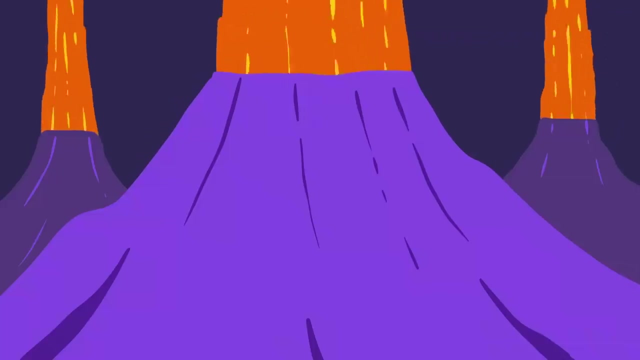 This newly exposed rock absorbed more carbon dioxide from rainfall, eventually removing so much atmospheric CO2 that the planet was plunged into a period called Snowball Earth. Over time, volcanic activity released enough CO2 to melt this ice, but that process took another 4 to 6 million years. Meanwhile, when the next supercontinent assembles, it's more likely to break down. Meanwhile, when the next supercontinent assembles, it's more likely to break down. Meanwhile, when the next supercontinent assembles, it's more likely to break down.